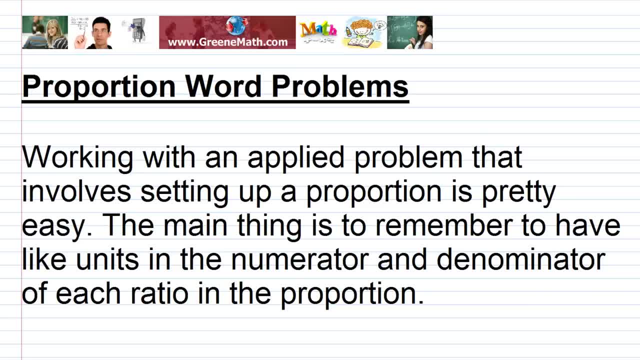 you're going to face in an Algebra 1 course. So the main thing that you have to remember is just to have like units in the numerator and denominator of each ratio in the proportion. And as we work through these sample problems, I'm going 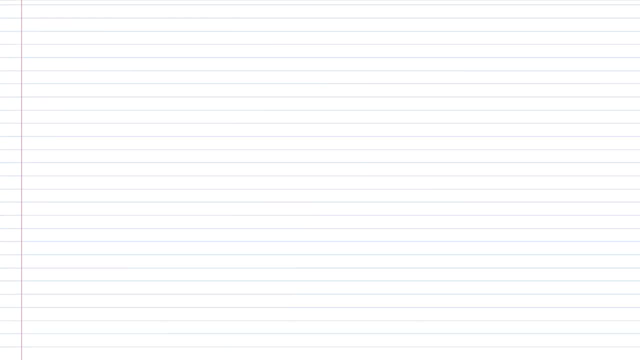 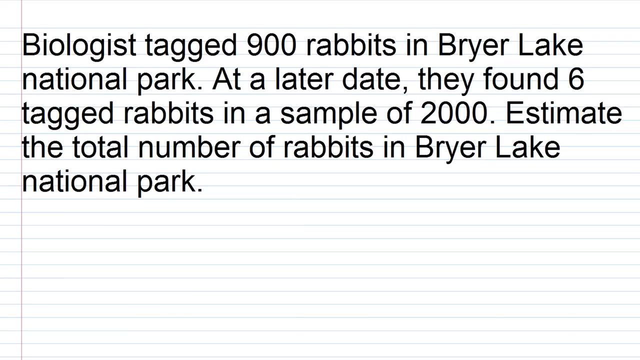 to explain that to you. So let's go ahead and look at the first problem here. Okay, so biologists tagged 900 rabbits in Briar Lake National Park. At a later date they found six tagged rabbits in a sample of 2,000.. Estimate the total. 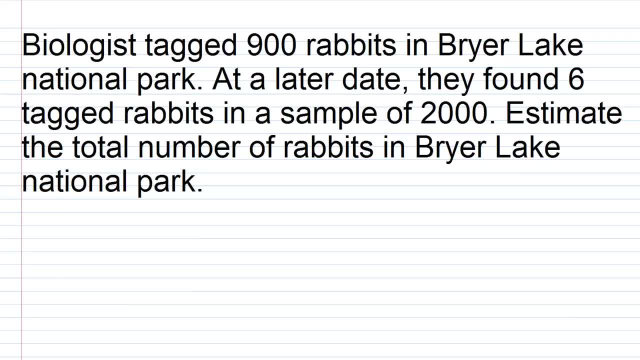 number of rabbits in Briar Lake National Park. So we're going to set up a proportion to perform this function here, which is to estimate the total number of rabbits in Briar Lake National Park. So let me set this one up for you, and then I'll kind. 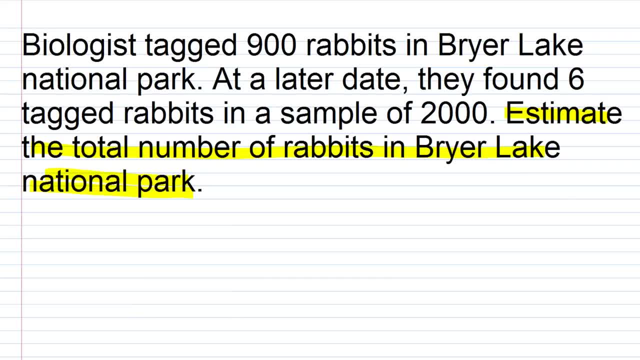 of go through it and explain. We're told in the problem here that biologists tagged 900 rabbits in Briar Lake National Park. So let's start with that. I'm just going to write 900, and then I'm just going to write tagged. 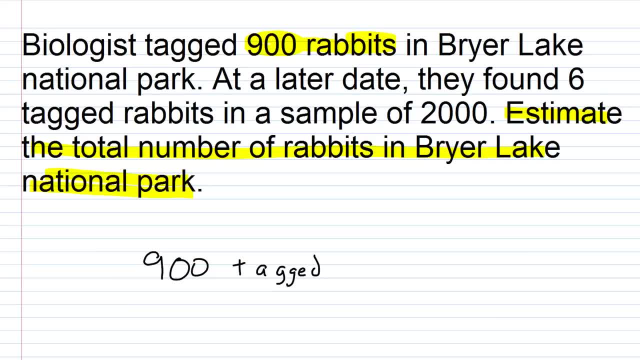 Okay, then we're told that at a later date they found six tagged rabbits. six tagged rabbits in a sample of 2,000.. Okay, in a sample of 2,000.. So here we have six tagged rabbits. I'm going to write six tagged and then I'm going to put this: 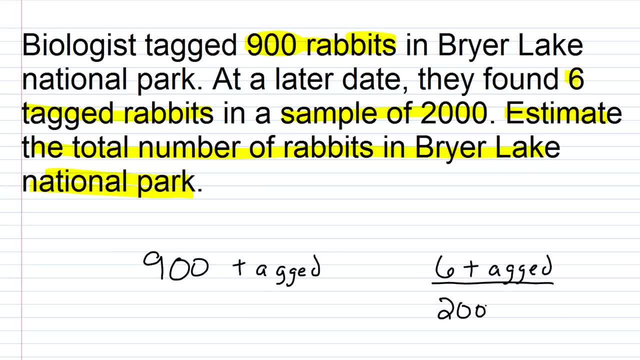 over the sample, which is 2,000.. I'll just put this as So. if we were to set these two equal to each other, we would be missing the denominator down here, which I could just represent with a variable like x, So the. 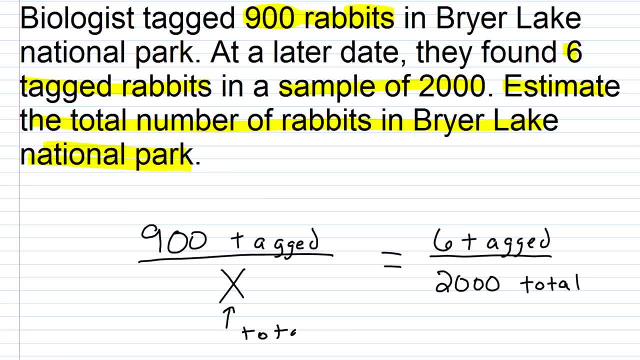 missing component. here is the total, which is exactly what's being asked in this question: Estimate the total number of rabbits in Briar Lake National Park. Now again, this is an estimate. It's not going to give us the exact number. If there was an exact number, this is a fictional problem. But let's go through and solve the proportion and we'll be able to do that. 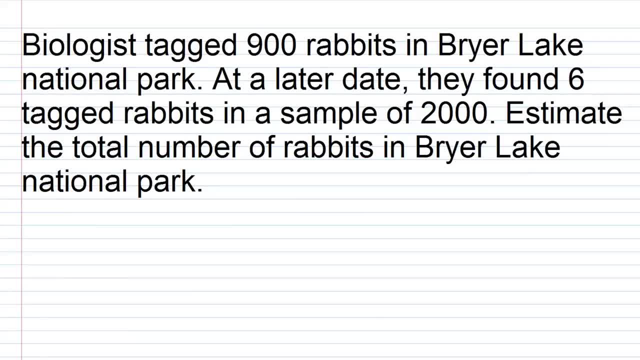 Estimate the total number of rabbits in Briar Lake National Park. So we're going to set up a proportion to perform this function here, which is the number of rabbits in Briar Lake National Park. So we're going to set up a proportion to perform this function here. 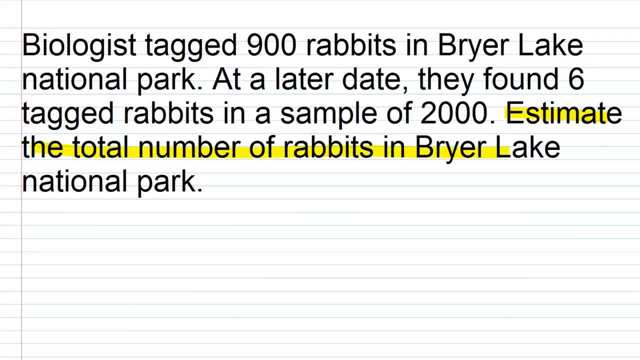 which is to estimate the total number of rabbits in Briar Lake National Park. So let me set this one up for you and then I'll kind of go through it and explain. We're told in the problem here that biologists tagged 900 rabbits in Briar Lake National Park. 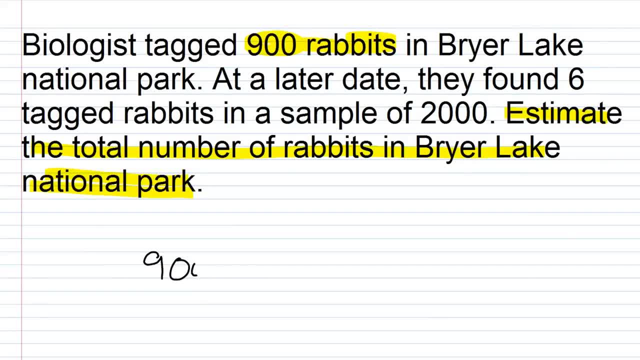 So let's start with that. I'm just going to write 900, and then I'm just going to write tagged. Okay, Then we're told that at a later date they found 6 tagged rabbits in a sample of 2,000.. 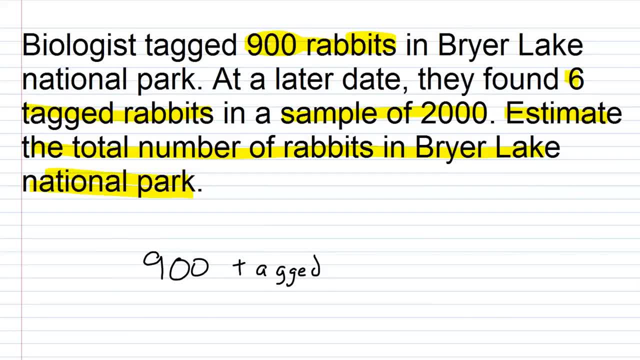 Okay, in a sample of 2,000.. So here we have 6 tagged rabbits. I'm going to write 6 tagged and then I'm going to put this over the sample, which is 2,000.. I'll just put this as: 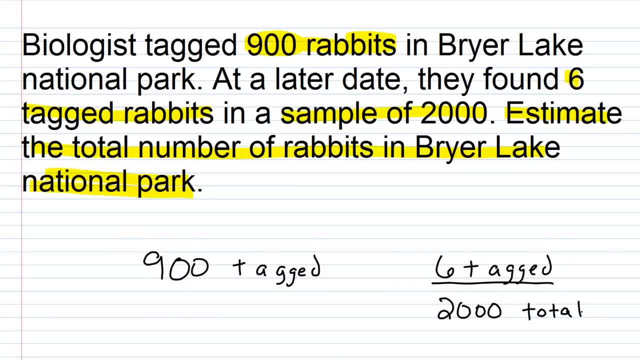 So if we were to set these two equal to each other, we would be missing the denominator down here, which I could just represent with a variable like x. So the missing component here is the total, which is exactly what's being asked in this question. 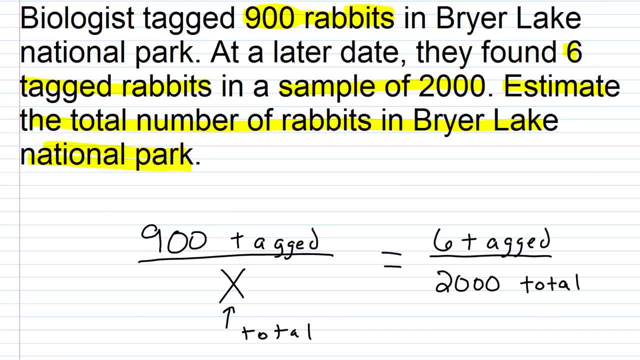 Estimate the total number of rabbits in Briar Lake National Park. Now again, this is an estimate. It's not going to give us the exact number. If there was an exact number, this is a fictional problem. But let's go through and solve the proportion and we'll be able to do that. 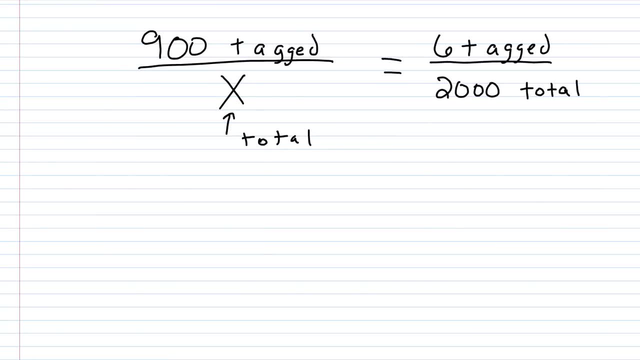 So to solve this again, we talked about how to solve a proportion. We're just going to cross multiply. I'm going to multiply 900 times 2,000.. So to do that quickly, it's 9 times 2,, that's 18.. 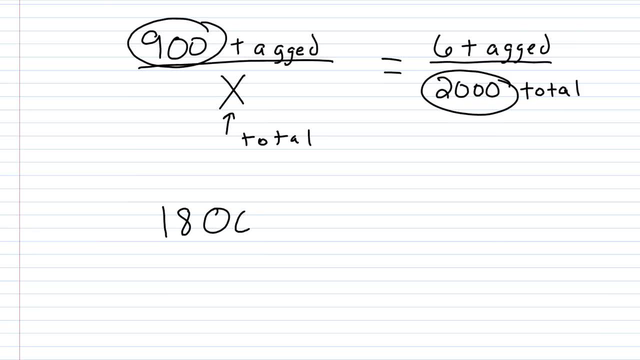 And then I have 1,, 2,, 3,, 4, 5 zeros: 1,, 2,, 3.. So that would be 1.8 million or 1,800,000.. And this would be equal to this times this 6x. 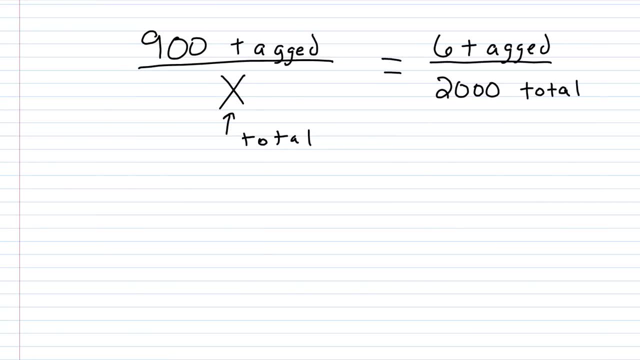 So to solve this again, we talked about how to solve a proportion. We're just going to cross, multiply. I'm going to multiply 900 times 2,000.. So to do that quickly, it's 9 times 2,, that's 18.. And then I have 1,, 2,, 3,, 4, 5 zeros. 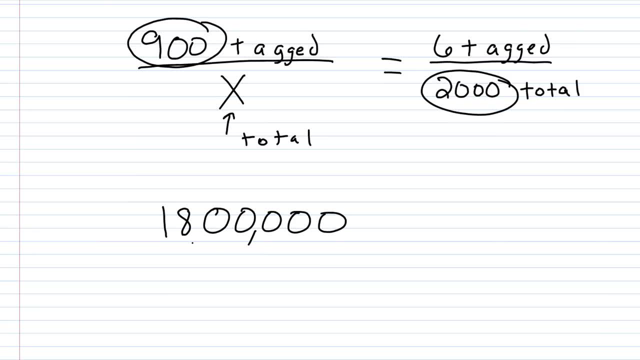 1, 2,, 3,, 4,, 5.. So that would be 1.8 million or 1,800,000.. And this would be equal to this times this 6x. So to solve this, we just divide both sides of the equation by 6. That. 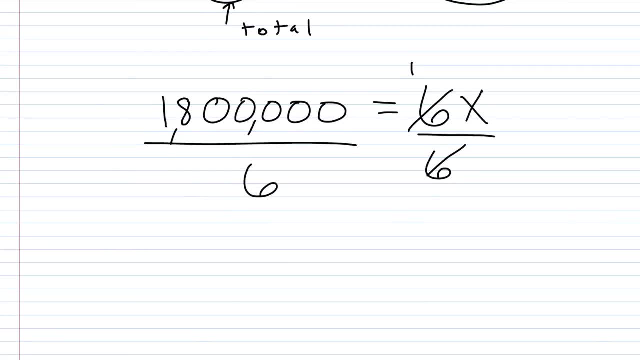 will become 1.. And then to do this, what we can do is divide 18 by 6.. That will give us 3.. And then we attach the zeros 1, 2, 3,, 4, 5,, so 1,, 2, 3, 4, 5,. so we get: x is equal to 300,000.. 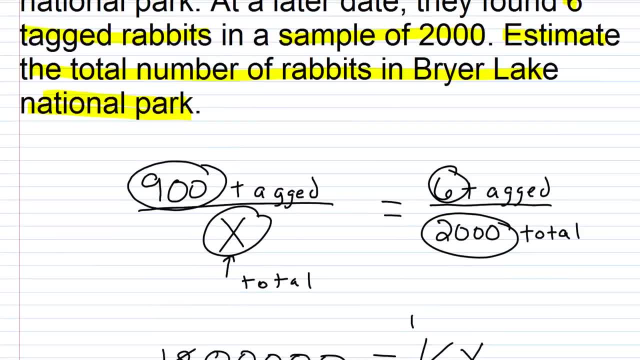 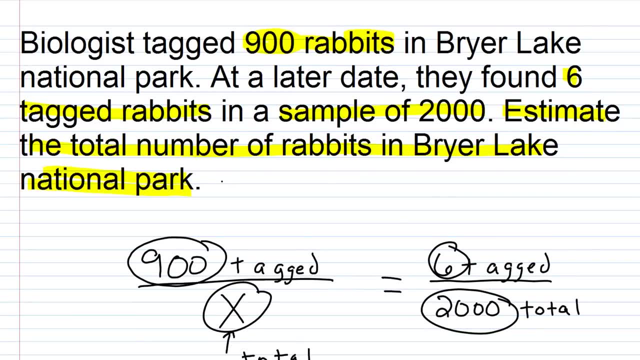 So if we scroll back up here, we can kind of make a nice little sentence for our problem here and just say that we estimate a total of 300,000 rabbits in Briar Lake National Park. So is that answer reasonable? if you wanted to check this. 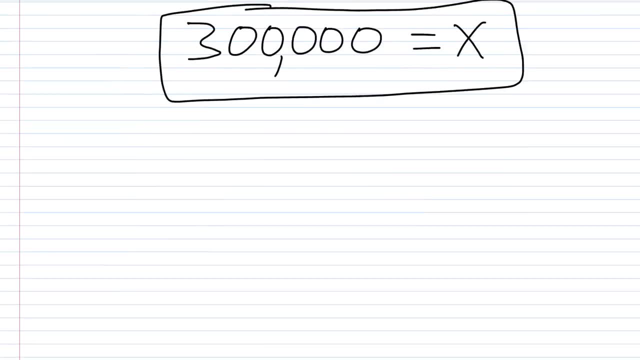 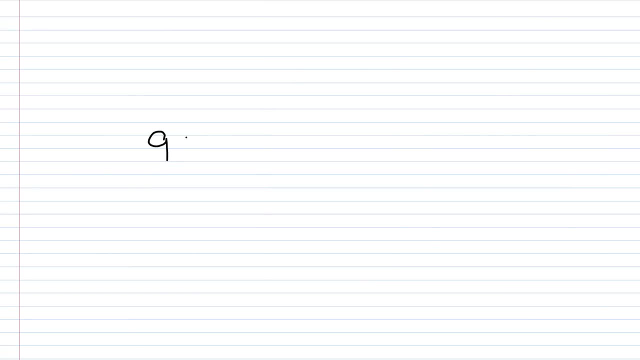 Well, let's see- I'm going to just check our proportion to make sure that's true- If, again, we have 900 rabbits that are tagged initially, and that's out of a total population of 300,000,. that's what we found. 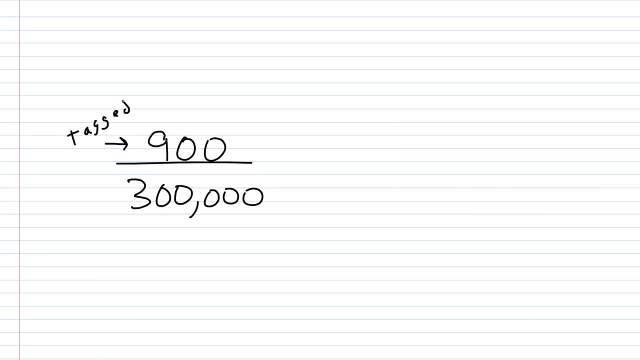 So again, this is the tagged number and this is the total population, And this is equal to what we find when we do a sample, which was 6 tagged rabbits and then a total population for the sample, of 2,000.. 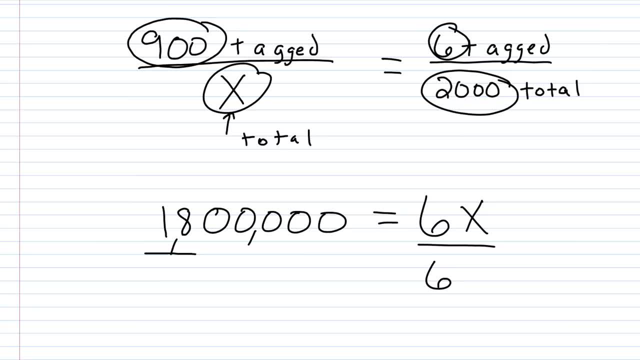 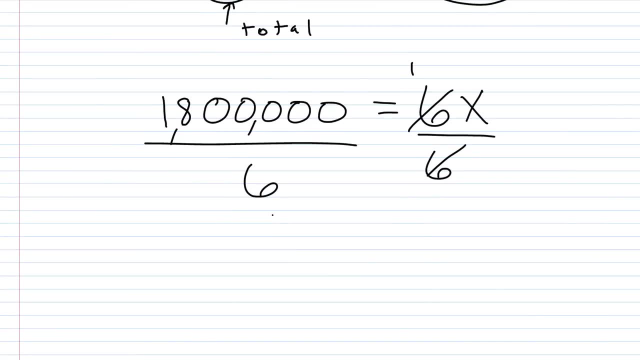 So to solve this, we just divide both sides of the equation by 6. That will become 1.. And then, to do this, what we can do is divide 18 by 6. That would give us 3.. And then we attach this: 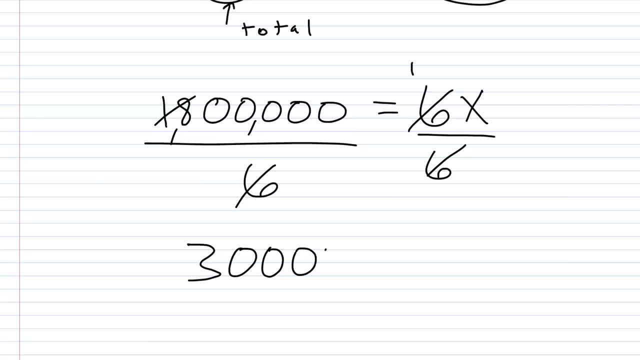 The zero is 1,, 2,, 3,, 4, 5.. So 1, 2,, 3,, 4, 5.. So we get: x is equal to 300,000.. So if we scroll back up here, 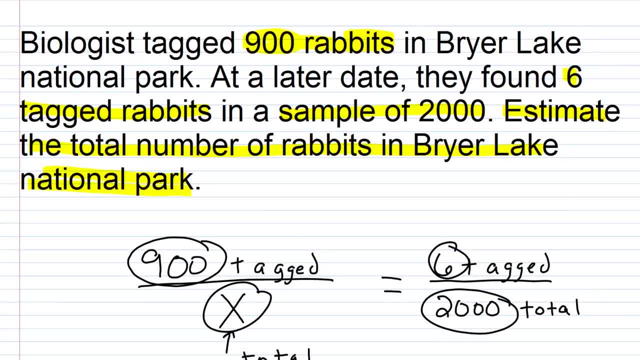 we can kind of make a nice little sentence for our problem here And just say that We estimate A total Of 300,000 rabbits in Briar Lake National Park. So is that answer reasonable? if you wanted to check this. 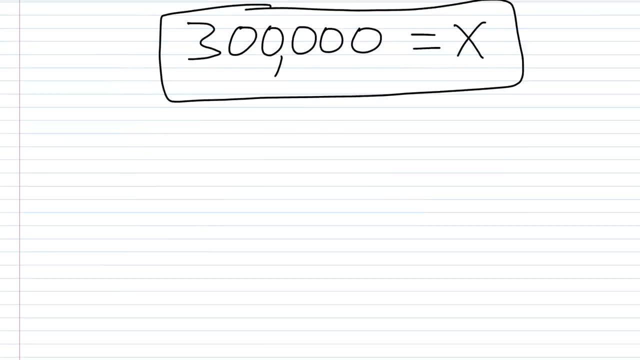 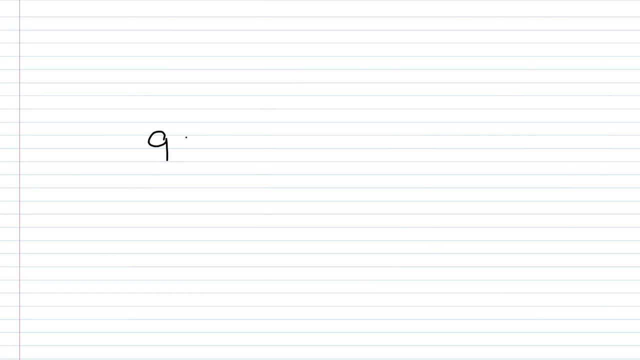 Well, let's see. We're going to just check our proportion to make sure that's true. So if again we have 900 rabbits that are tagged initially, and that's out of a total population of 300,000, that's what we found. so again, this is the tagged number and 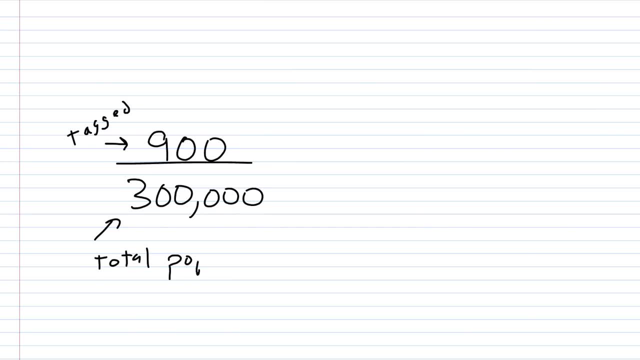 this is the total population and this is equal to what we find when we do a sample, which was 6 tagged rabbits And then a total population for the sample of 2,000.. These two ratios should be equal and if they are, we should have the right answer. 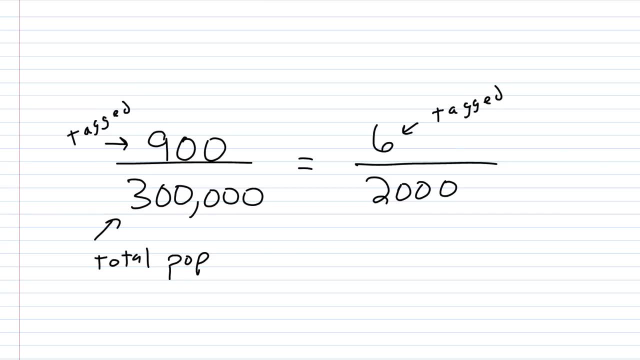 Now remember again: I said that this would be an estimate. So if this was a real problem, you wouldn't have exactly 300,000 rabbits, but you would have. you would expect to have something close to that number. 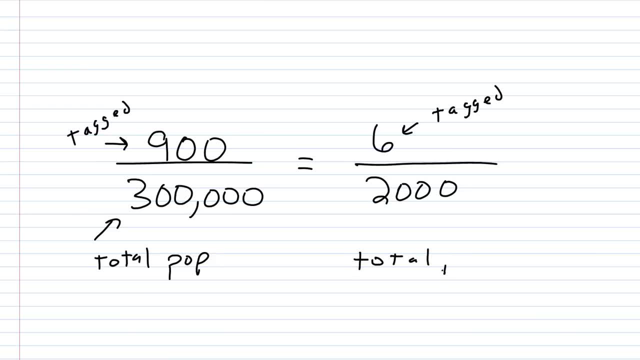 So notice how the units here Match up. The numerators both represent the number of tagged rabbits, and the denominators both represent the numbers that we're using to represent the total population. Now again, on this one we're talking about the sample population, and on this one we're 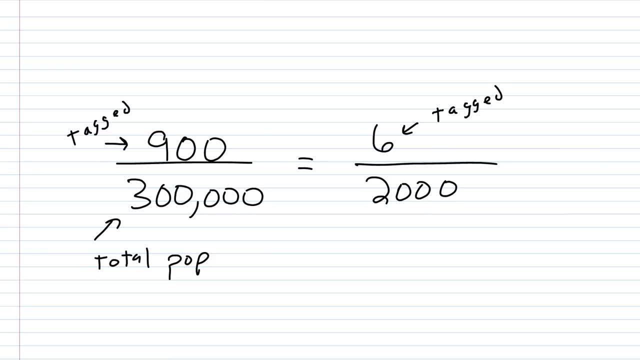 These two ratios should be equal and if they are, we should have the right answer. Now remember again: I said that this would be an estimate, So if this was a real problem, you wouldn't have exactly 30. So again, I'm going to check our proportion to make sure that's true. So again, I'm going to check our proportion to make sure that's true. So again, I'm going to check our proportion to make sure that's true. But I don't think we're going to have 500 or 300,000 rabbits. 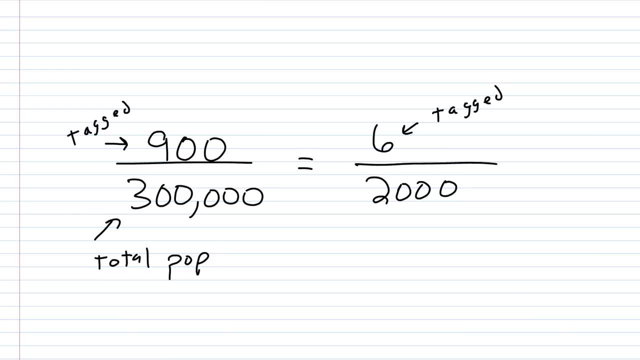 But you would have. you would expect to have something close to that number. So notice how the units here match up. The numerators both represent the number of tagged rabbits and the denominators both represent the numbers that we're using to represent the total population. 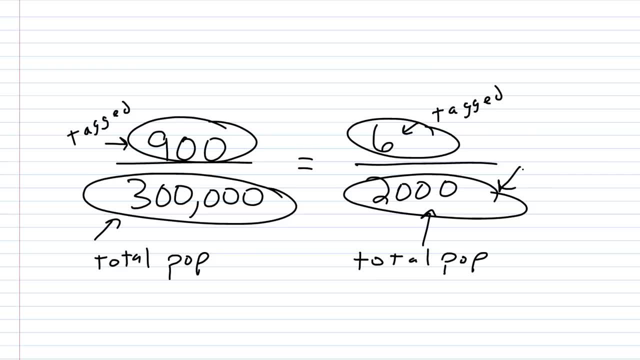 Now again, on this one we're talking about the sample population and on this one we're talking about the total population. All right, So if we click on the save, we're going to have a really 1965 – über 30,000 – 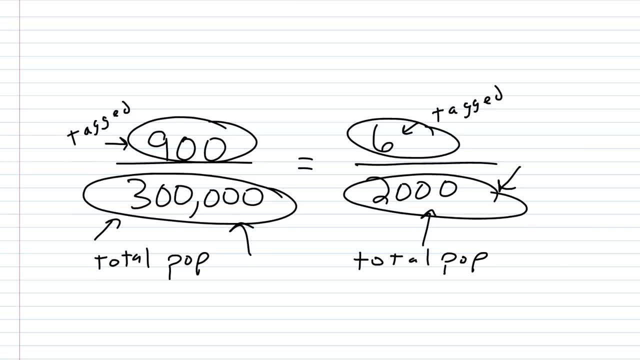 cross-multiply here: 300,000 times 6,, we know that's 1.8 million. and then 2,000 times 900, that's also 1.8 million. So these two sides are equal and that tells me we have the correct. 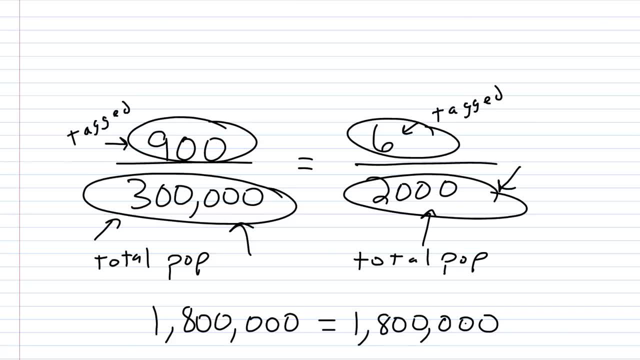 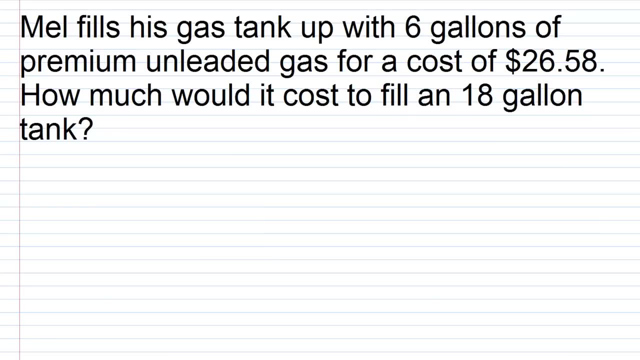 answer. Okay, here's another easy one. Mel fills his gas tank up with six gallons of premium unleaded gas for a cost of $26.58.. How much would it cost to fill an 18-gallon tank? So for this one again, we're just going to set up a quick little proportion. 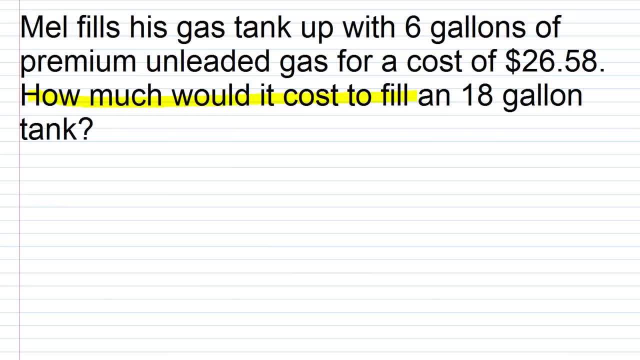 And the main question we're trying to answer here is: how much would it cost to fill an 18-gallon tank? So right here we're given that he fills up his gas tank with six gallons of gas and we're given the cost of that six gallons: $26.58.. So we'll start with the ratio. 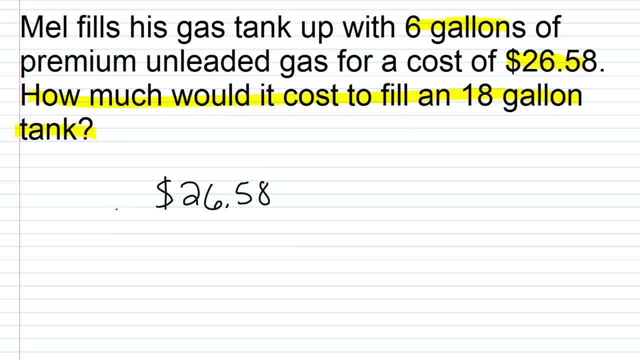 $26.58.. This would be the cost And then in the denominator we'll put how many gallons he got, for. that cost six gallons, Then we're going to set this equal to. we want to know how much it would cost to fill an 18-gallon. 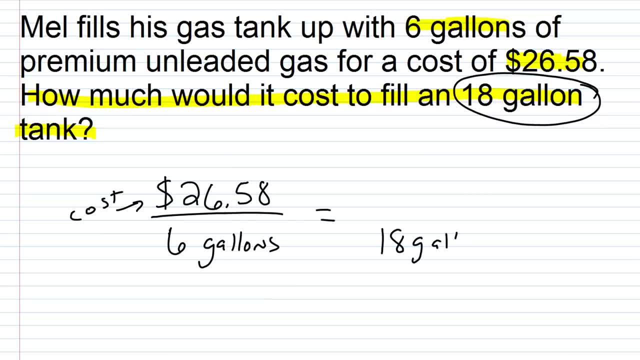 tank, So we'll have 18 gallons down here. This will give you the same units in the denominators. And then the unknown here is the cost, right, because that's what we're trying to find. So we just represent this unknown with a variable, so we'll just put x here. 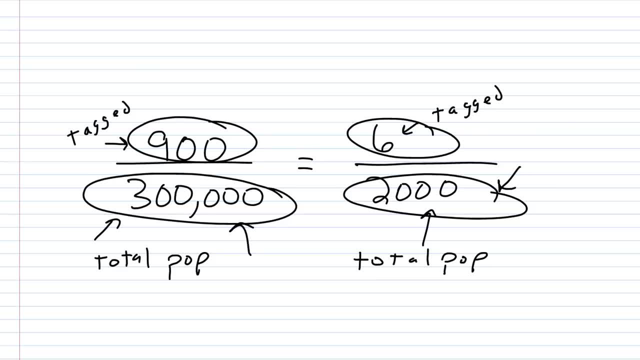 talking about the total population. Alright, so if we cross, multiply here 300,000 times 6,, we know that's 1.8 million, and then 2,000 times 900, that's also 1.8 million. 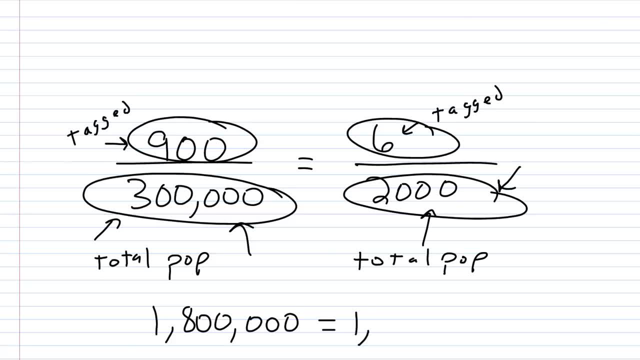 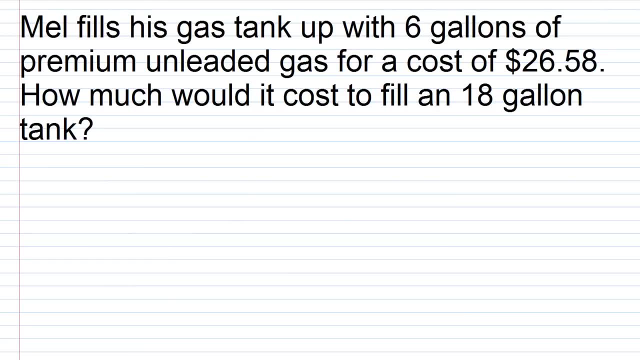 So these two sides are equal And that tells me we have the correct answer. Okay, here's another easy one. Mel fills his gas tank up with 6 gallons of premium unleaded gas for a cost of $26.58.. How much would it cost to fill an 18-gallon tank? 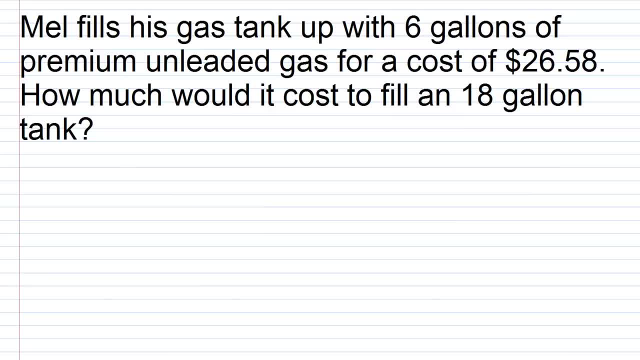 So for this one again, we're just going to set up a quick little proportion, And the main question we're trying to answer here is: how much would it cost to fill an 18-gallon tank? So right here we're. given that he fills up his gas tank with 6 gallons of gas and 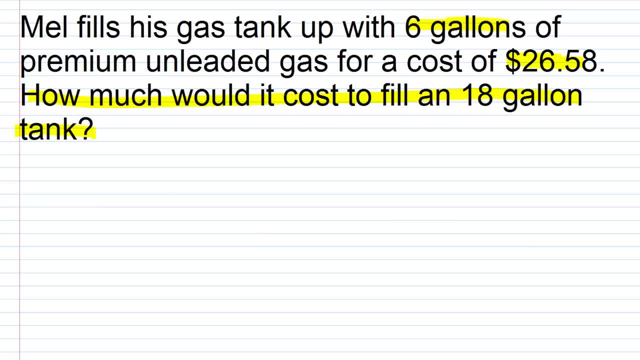 we're given the cost of that 6 gallons $26.58.. So we'll start with the ratio $26.58, this would be the cost, and then in the denominator we'll put how many gallons he got, for that cost 6 gallons. 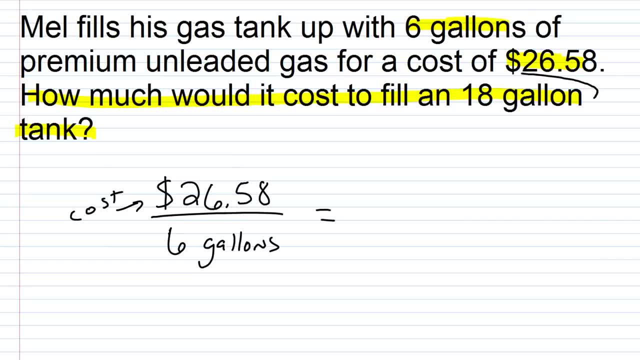 Then we're going to set this equal to. we want to know how much it would cost to fill an 18-gallon tank, so we'll have 18 gallons down here. this will give you the same units in the denominators, and then the unknown here is the cost. right, because that's what. 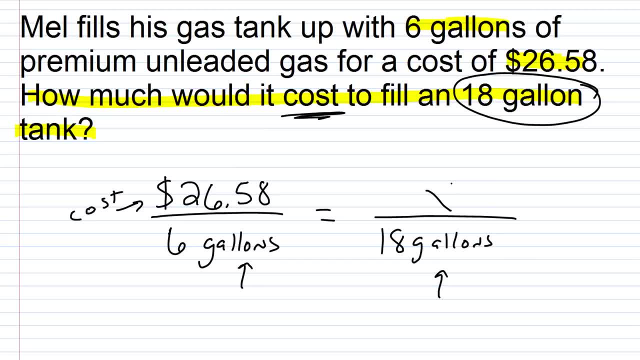 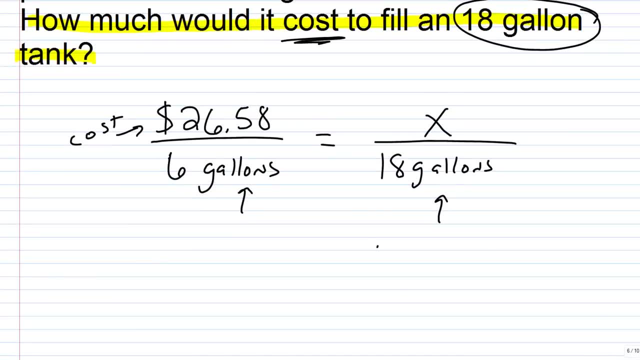 we're trying to find. So we just represent this unknown with a variable. so we'll just put x here and then we'll just do some cross-multiplying and we'll solve for x. So we'll have 6 times x. that's: 6x equals 18 times 26.58, and if you punch that up on 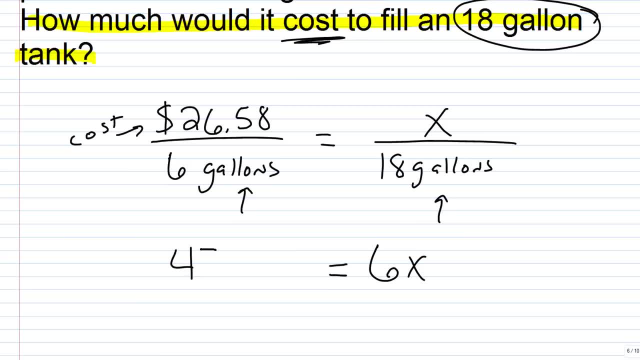 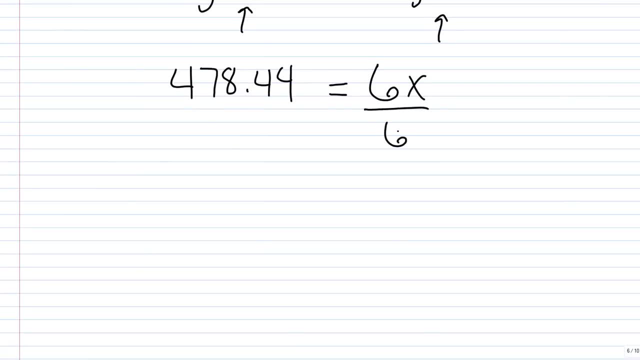 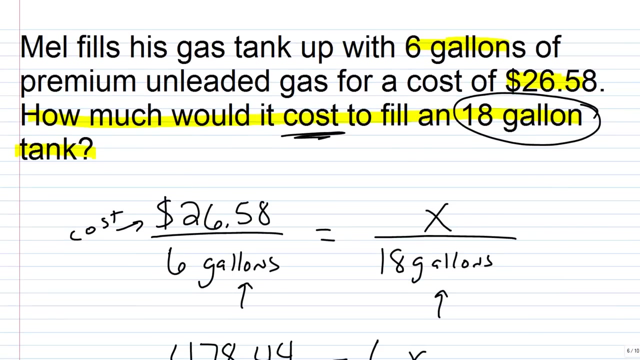 a calculator, you're going to get 478.44.. Now continuing, we just divide both sides of the equation by 6, and you're going to get x equals 79.74.. So this, right here, would be the cost to fill an 18-gallon tank. 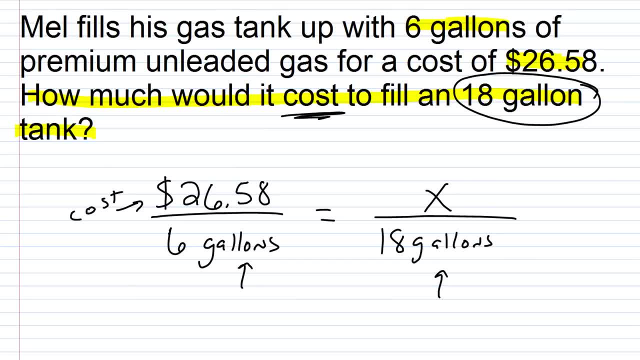 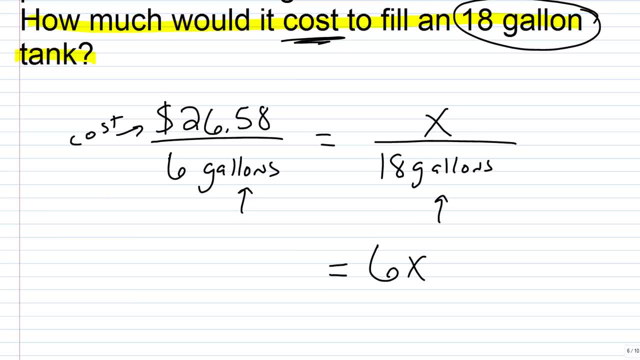 And then we'll just do some cross-multiplying and we'll solve it. So we'll have 6 times x. that's: 6x equals 18 times 26.58.. And if you punch that up on a calculator, you're going to get 478.44.. 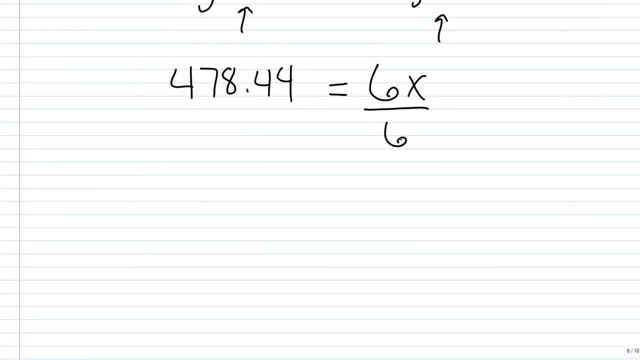 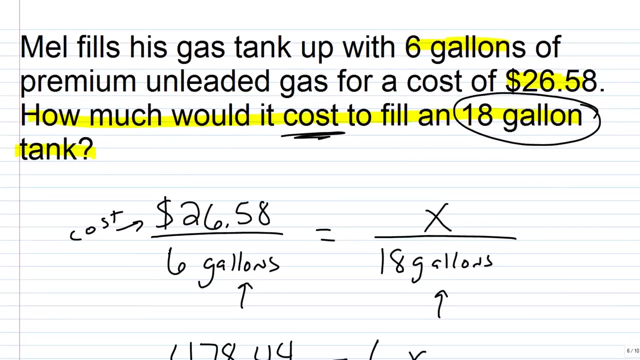 Now continuing, we just divide both sides of the equation by 6, and you're going to get x equals 79.74.. So this, right here, would be the cost To fill an 18-gallon tank. just write a little sentence here: it would cost. 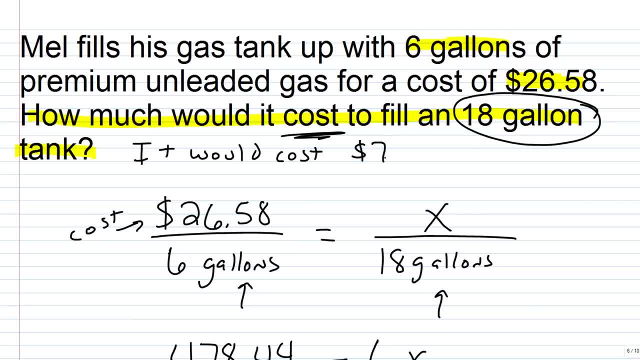 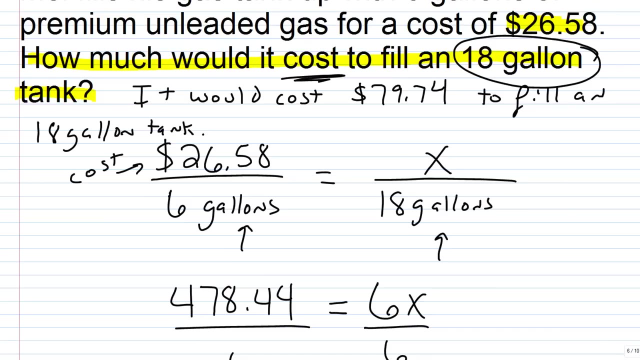 $79.74 to fill an 18-gallon tank. Now one way you can check this is just to figure out the unit rate here. If you divide 26.58, by 6,, you get 4.43.. So that means you're paying $4.43 per gallon. 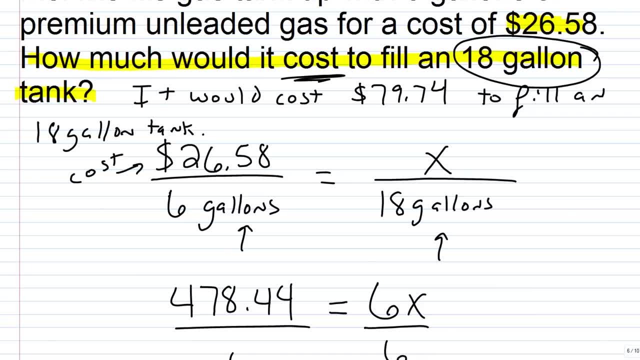 Now, if you have that same unit rate and you multiply that 4.43 times 18,, you end up with $79.74.. And that's what we got for the answer to the problem. So we know here the answer is going to be correct. 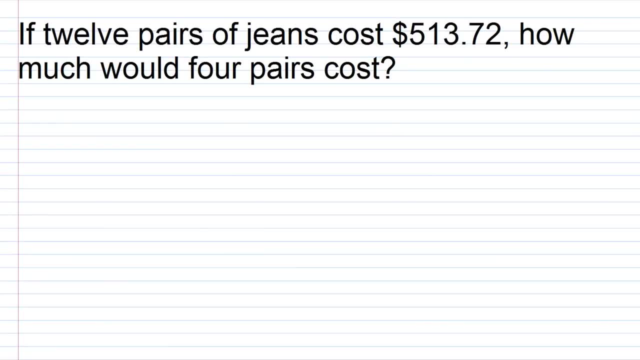 OK, if 12 pairs of jeans cost $513.72,, how much would 4 pairs cost? So again another easy one: 12 pairs- so I'm going to highlight 12 here- cost $513.72.. And then the main thing: how much would 4 pairs cost? 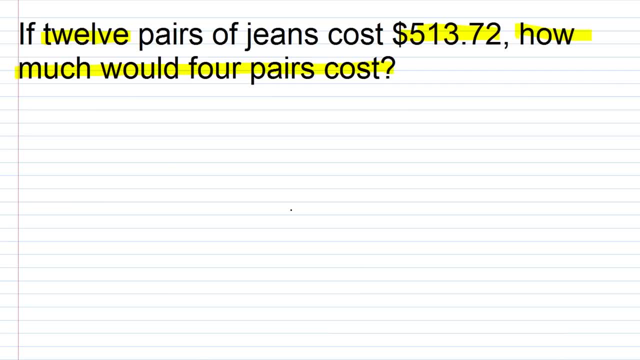 So we can basically do the exact same thing we did in the last problem. You have your cost- $513.72, over your quantity, which is 12.. And you set this equal to what you need to figure out. Now you're given the quantity that you're going to need to figure out. 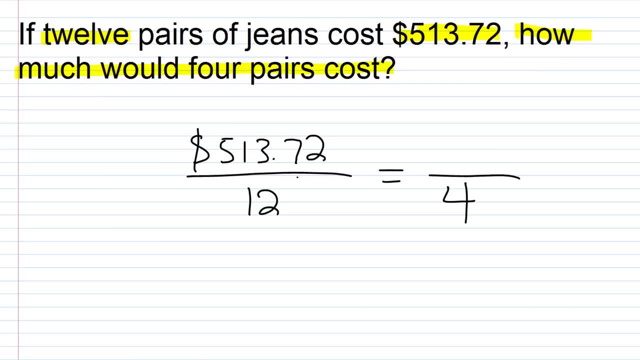 The quantity that you're looking for, which is 4.. And you want to know the cost, which is going to be x, That's your unknown. Same units in the numerators, Same units in the denominators. We crossmultiply and set this up. 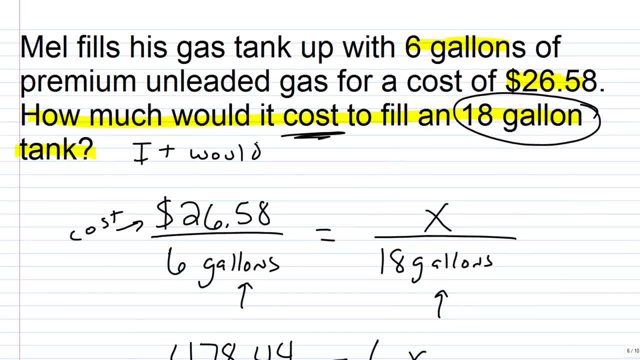 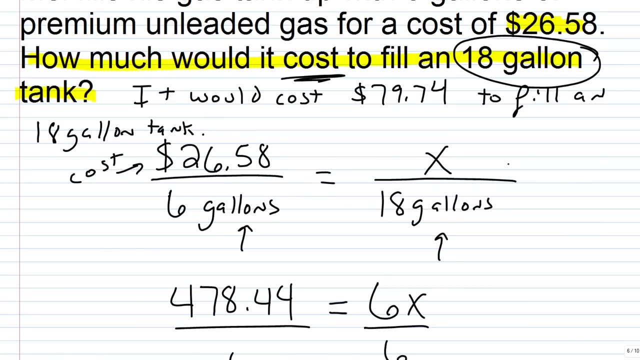 Just write a little sentence here: It would cost $79.00.. $79.74 to fill an 18-gallon tank. Now, one way you can check this is just to figure out the unit rate here. If you divide 26.58 by 6,, you get 4.43.. 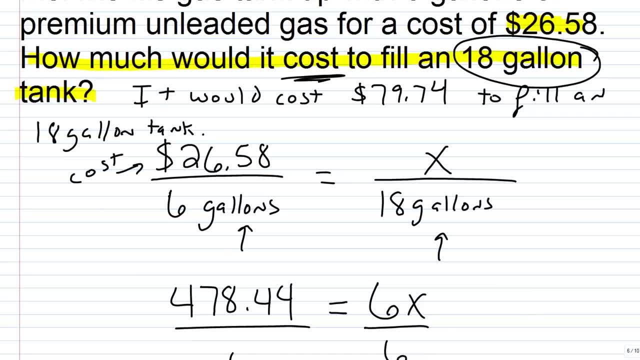 So that means you're paying $4.43 per gallon. Now, if you have that same unit rate and you multiply that by 6,, you're going to get $4.43.. And you multiply that 4.43 times 18,, you end up with $79.74.. 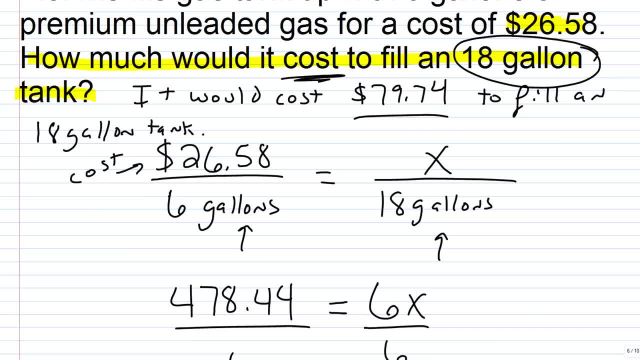 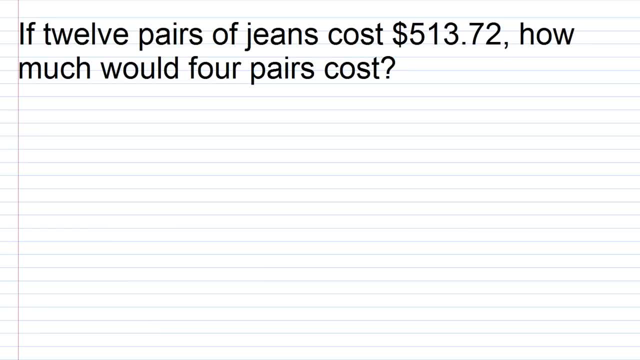 And that's what we got for the answer to the problem. So we know here the answer's going to be correct. Okay, if 12 pairs of jeans cost $513.72,, how much would 4 pairs cost? So again, another easy one. 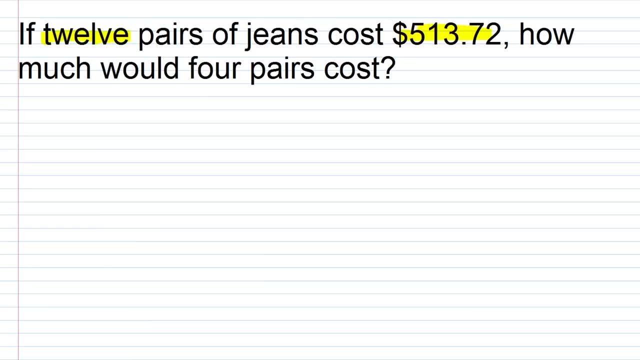 12 pairs- so I'm going to highlight 12 here- cost $513.72.. And then the main thing: how much would 4 pairs cost? So we can basically do the exact same thing we did in the last problem. 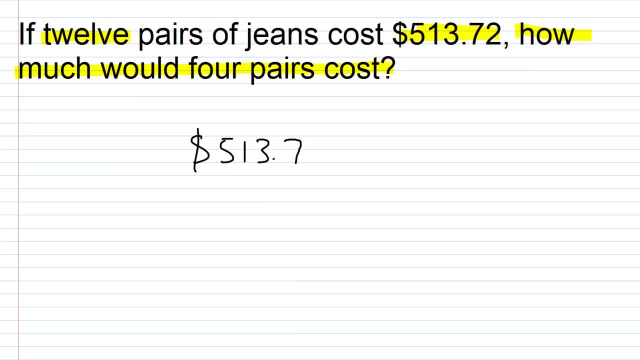 You have your cost- $513.72, over your quantity, which is 12.. And you set this equal to what you need to figure out. Now you're given the quantity that you're looking for, which is 4.. And you want to know the cost, which is going to be x. 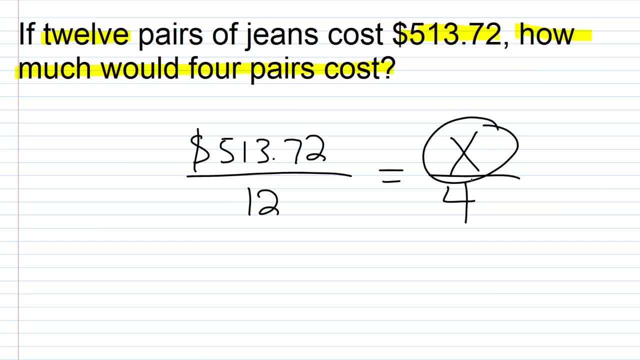 That's your unknown. Same units in the numerators, Same units in the denominators. We cross-multiply and set this up: 12 times x is 12x. 4 times 513.72 is 2,054.88.. 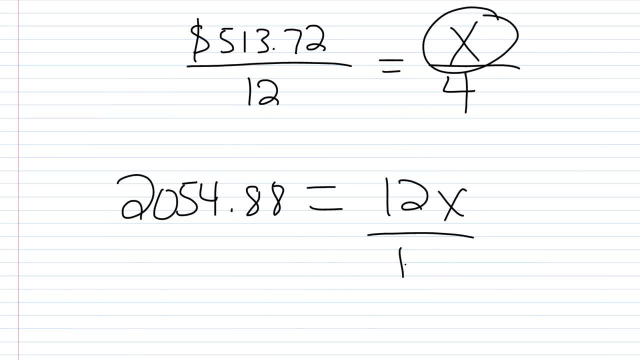 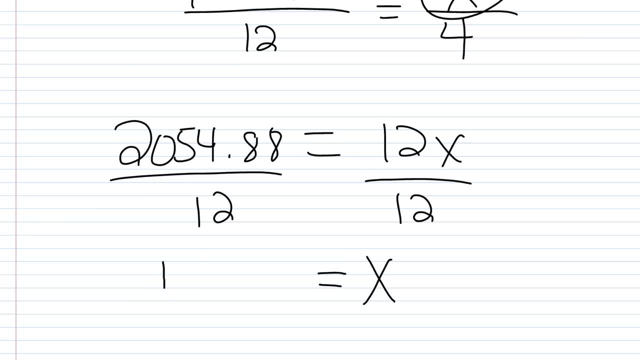 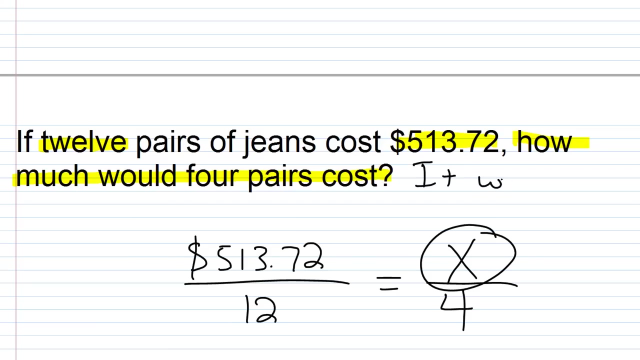 Now we're going to divide both sides of this equation by 12.. And you're going to get x equals 171.24.. So $171.24 would be your cost for 4 pairs of jeans. So it would cost $171.24 for 4 pairs of jeans. 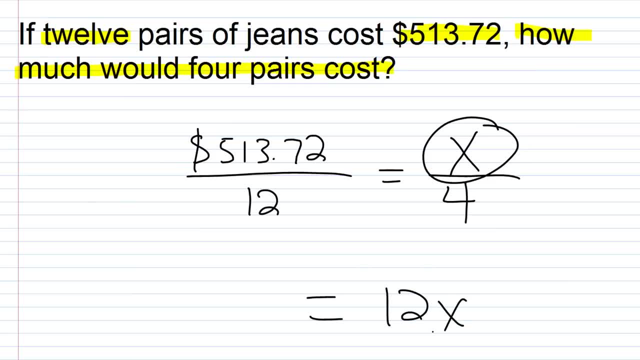 12 times x is 12 x 4 times 513.72 is $2,054.88.. Now we're going to divide both sides of this equation by 12, and then find two other units that are equal to $513.72.. And we get our $2015.68.. Now, talking about the three-dimensional equation, if you look at the meidän LIBRARIUM- sorry, there's only two hundred units and we have twelve. The second set of totals equals $18.49.. 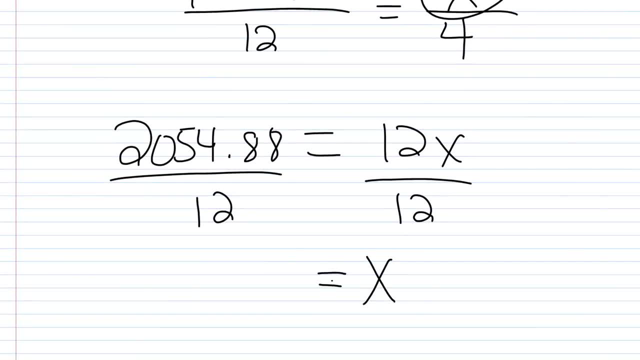 If you fill out that capital choice equation, you're going to get each set of 12 and the other the gross rupees you're going to get. x equals 171.24.. So $171.24 would be your cost for four pairs of genes. 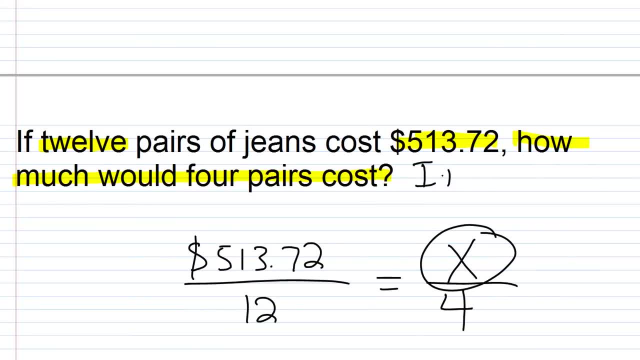 Okay, so it would cost $171.24 for four pairs of genes. Now again, if you want to check this, you could find the unit rate If you divide 513.72 by 12,. right, it's basically this. right here you get your unit rate. Here's your 42.81.. So, if you have, 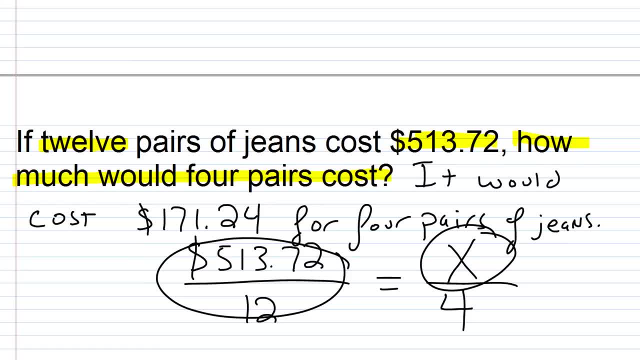 the correct answer. when you multiply 42.81 times 4,, you should get this number here, 171.24.. And if you do that on a calculator, you'll see that that's the number you do get. So you can either check it by plugging in the number that you get for x in your proportion. 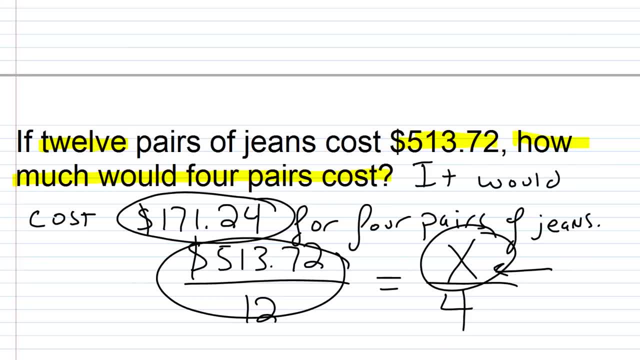 and you can check and cross multiply. make sure they're equal. That's one way to check. Or you can get the unit rate. Make sure the unit rates match. Okay, if the unit rates match, or if you cross, multiply and it's. 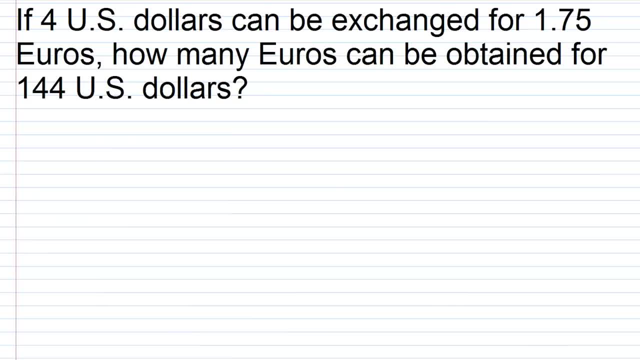 equal. either way, you know you have the correct answer. Okay, if four US dollars can be exchanged for 1.75 euros, how many euros can be obtained for 144 US dollars? So again, another easy one. So let's jump right into this. So four US dollars can be exchanged for 1.75 euros. 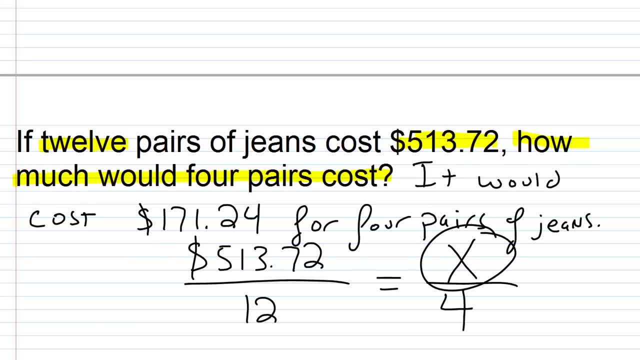 Now again, if you want to check this, you could find the unit rate If you divide 513.72 by 12,. right, It's basically this. right here You get your unit rate. Here's your 42.81.. 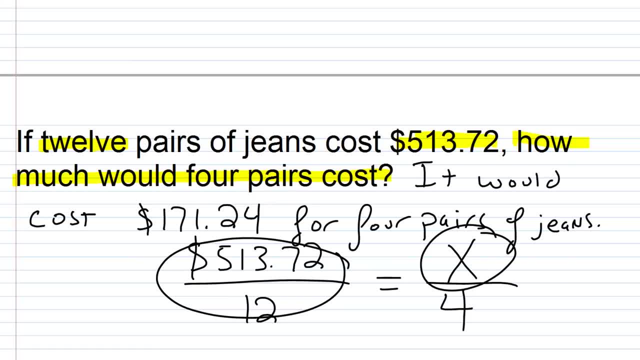 So if you have the correct answer, when you multiply 42.81 times 4,, you should get this number here 171.24.. And if you do that on a calculator, you'll see that that's the number you do get. 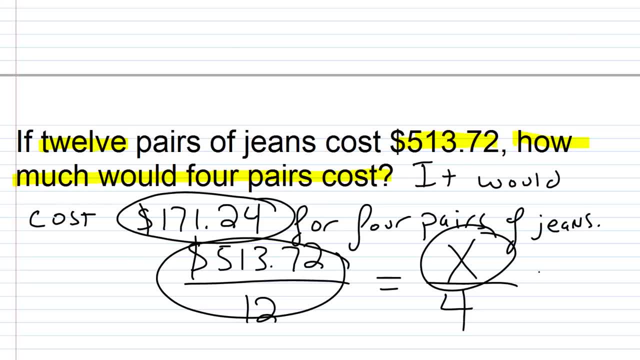 So you can either check it by plugging in The number that you get for x in your proportion And you can check, You can cross-multiply and make sure they're equal. That's one way to check. Or you can get the unit rate and make sure the unit rates match. 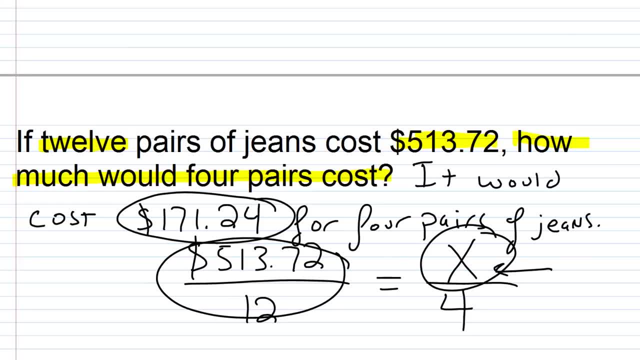 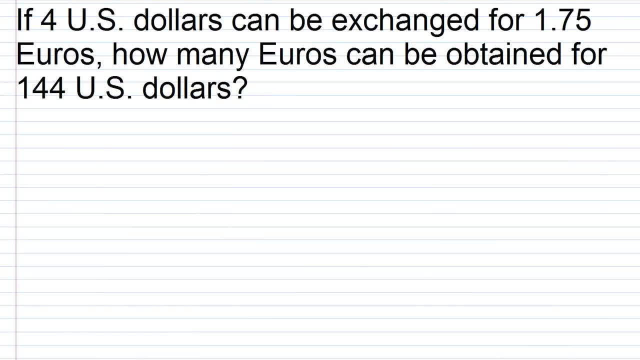 Okay, if the unit rates match or if you cross-multiply and it's equal. either way, you know you have the correct answer. Okay, If 4 US dollars can be exchanged for 1.75 euros, how many euros can be obtained for 144 US dollars? 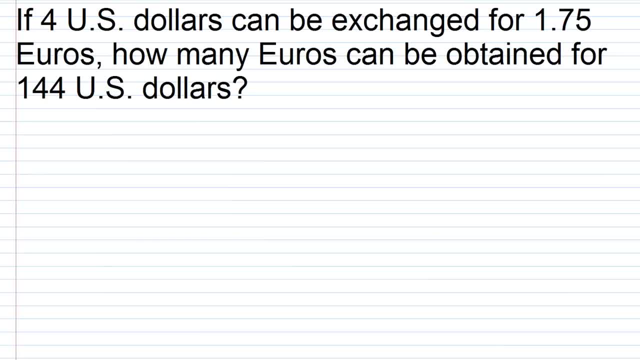 So I don't know, I don't know. Again, another easy one, So let's jump right into this. So 4 US dollars can be exchanged for 1.75 euros, So we can just write this as 4 dollars over 1.75 euros. 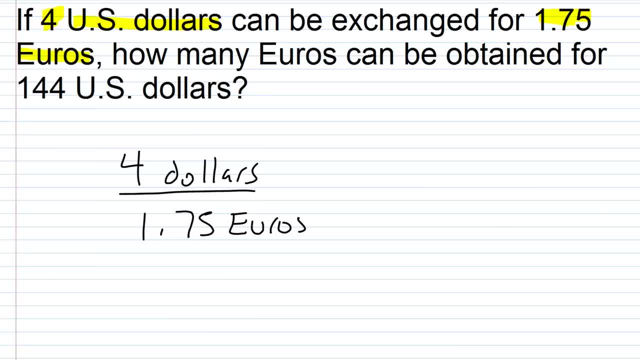 I'm going to show you, after we're finished here, that you can flip that And as long as you flip it in the other ratio that you're setting it equal to, you're going to get the same answer. So the main question here is: it asks how many euros can be obtained for 144 US dollars. 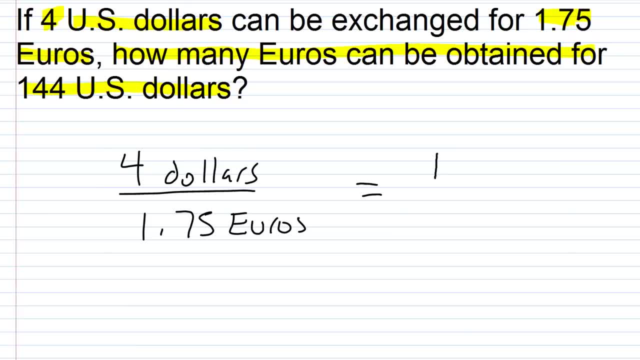 So dollars is in the numerator, So we're going to put dollars in the numerator, 144 dollars- And then we don't know at this point how many euros we can get for that. So we just put X. You can put X euros if you want. 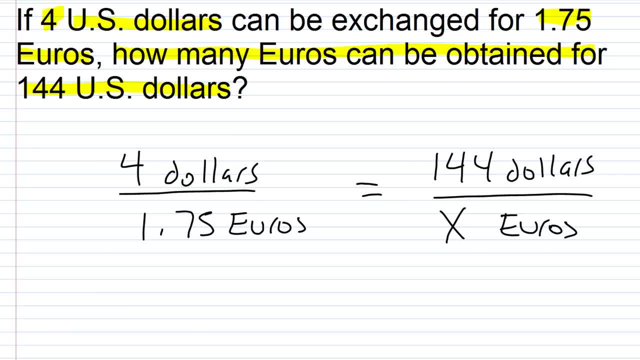 So the units match. Units and denominator match, The units and numerator match. So we're just going to cross multiply here and solve for X. If you take 144 and you multiply by 1.75, you will get 252.. 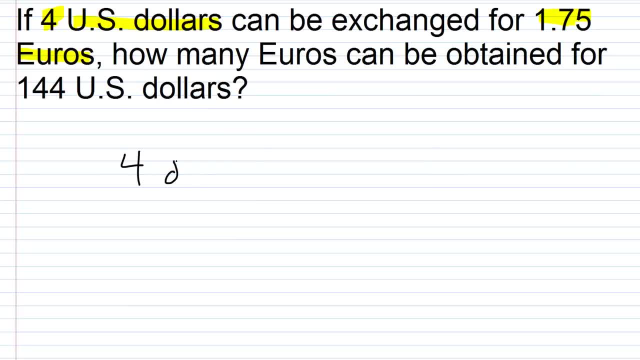 So we can just write this as: four dollars over 1.75 euros. I'm going to show you after we're finished here that you can flip that, and as long as you flip it in the other ratio that you're setting it equal to. 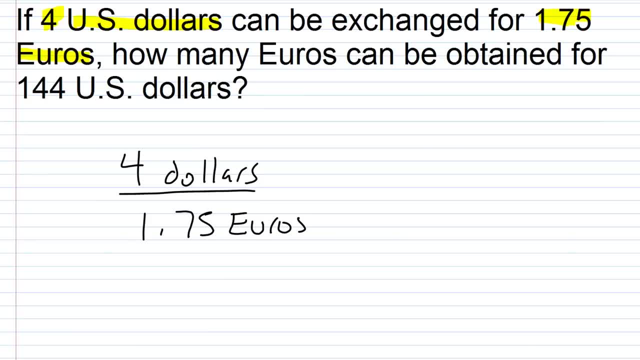 you're going to get the same answer. So the main question here is: it asks how many euros can be obtained for 144 US dollars. So dollars is in the numerator, so we're going to dollars in the numerator, $144.. And then we don't know at this point how many euros we can get for. 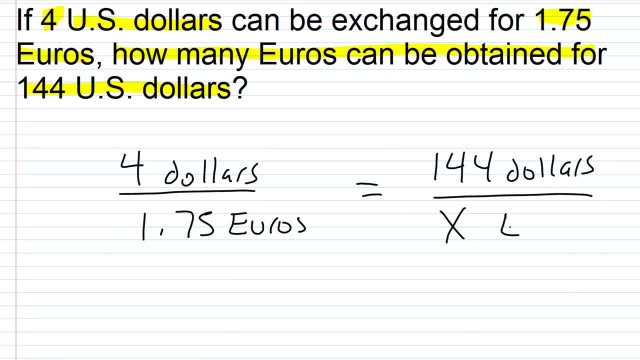 that. So we just put X. You can put X euros if you want. So the units match Units and denominator match, The units and numerator match. So we're just going to cross multiply here and solve for X. If you take 144 and you multiply by 1.75, you will get 252.. And then 4 times X is 4X. 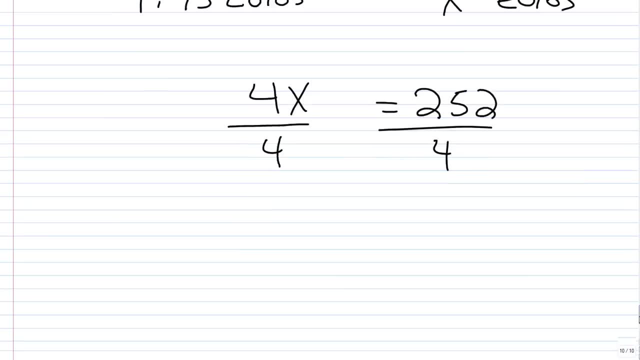 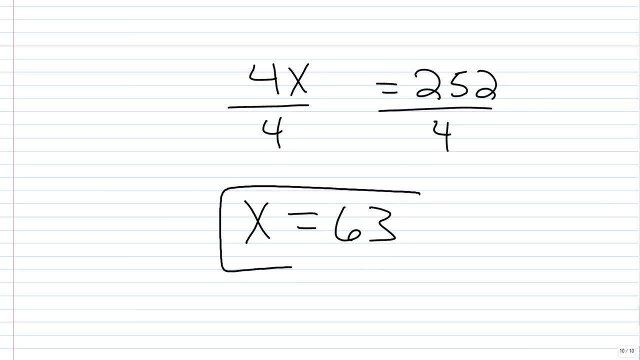 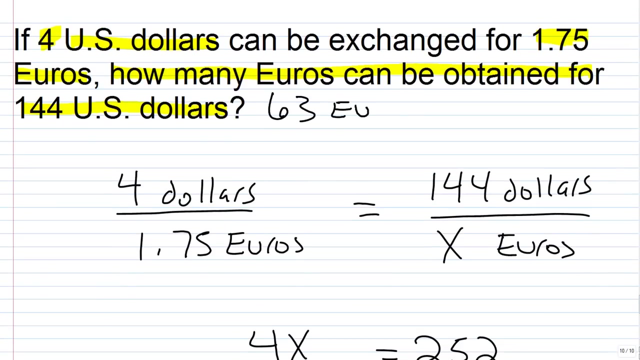 Divide both sides of the equation by 4. This will be: X equals 63. So that means you can get 63 euros. 63 euros Can be obtained for 144 US dollars, So finding the unit rate here really isn't a good way to check this. We would. 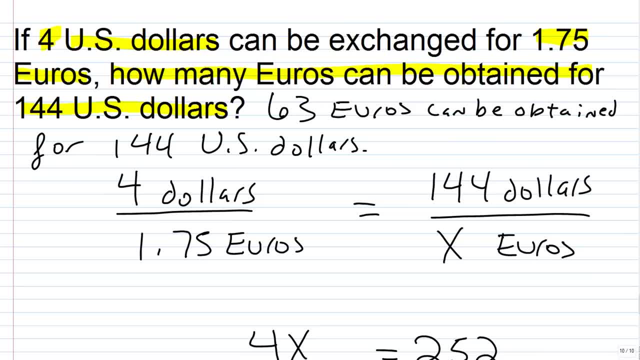 just go ahead and cross multiply. It's just because when you divide 4 by 1.75, you end up with a really funky decimal And I don't want to get into that right now. So let's just cross multiply to check. So we'll take 4 by 1.75.. We'll take 4 by 1.75.. We'll take 4 by 1.75.. 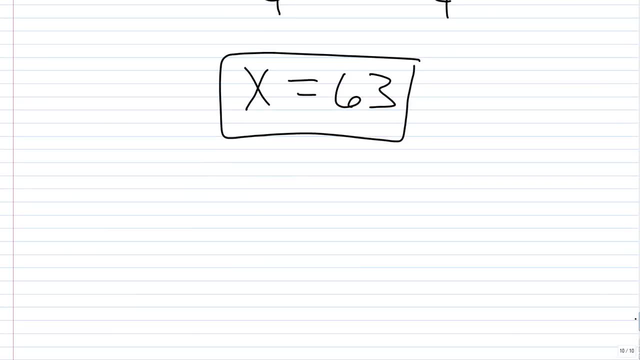 We'll take: 4 over 1.75 equals 144 over 63. So 63 times 4 is 252.. And we already know that 1.75 times 144 is also 252.. So this checks out. Now let me flip this and show you. 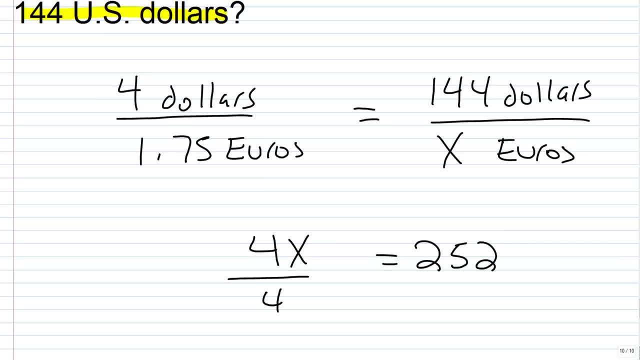 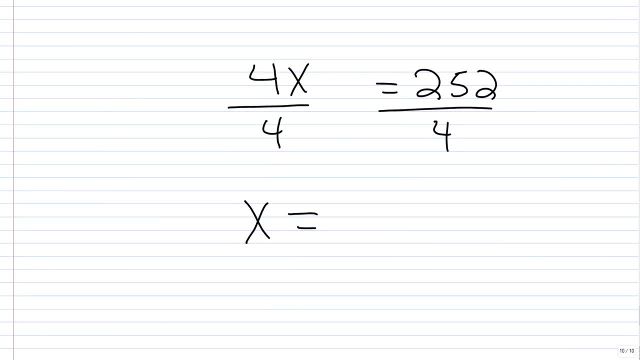 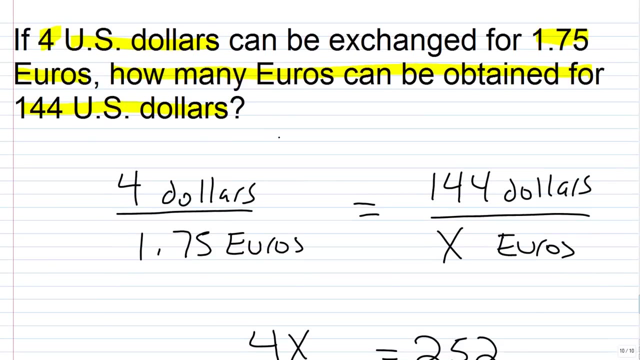 And then 4 times X is 4X. Divide both sides of the equation by 4. This will be X equals 63. So that means you can get 63 euros. 63 euros can be obtained for 144 US dollars. 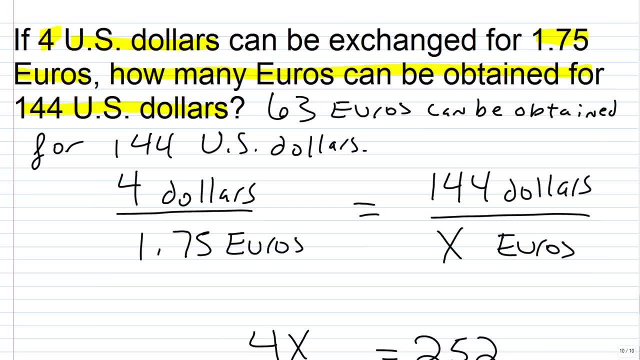 So finding the unit rate here really isn't a good way to check this. We would just go ahead and cross multiply. It's just because when you divide 4 by 1.75, you end up with a really funky decimal, And I don't want to get into that right now. 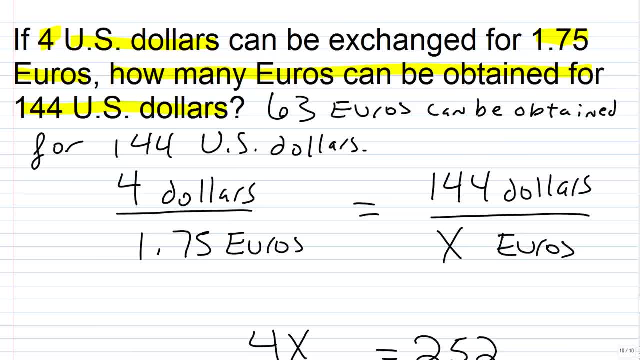 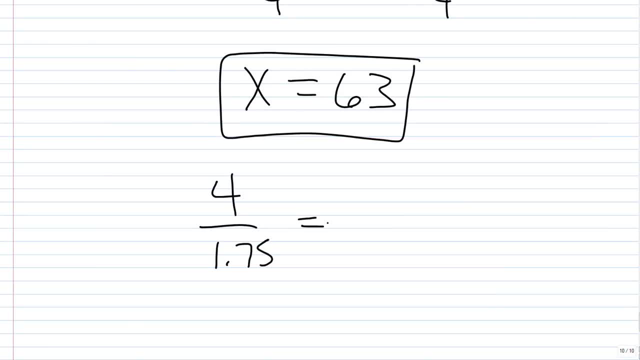 So let's just cross multiply to check. So we'll take: 4 over 1.75 equals 144 over 63.. So 63 times 4 is 252.. And we already know that 1.75 times 144 is also 252.. 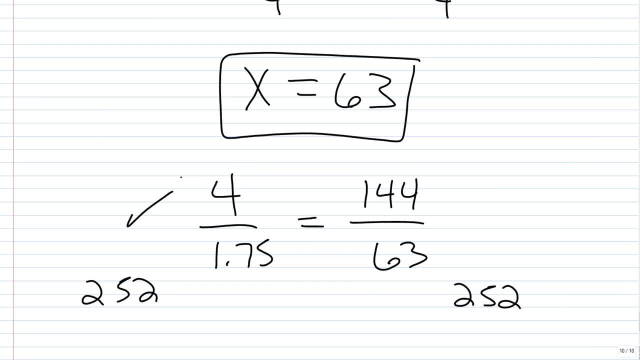 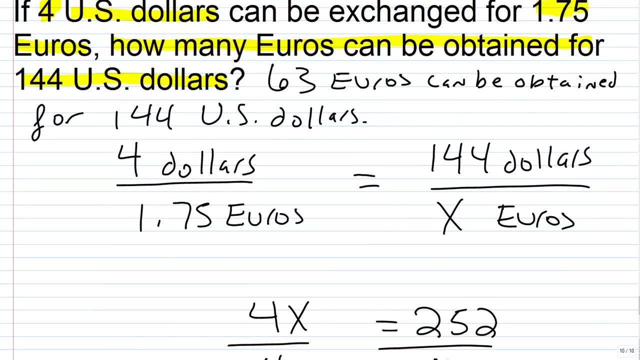 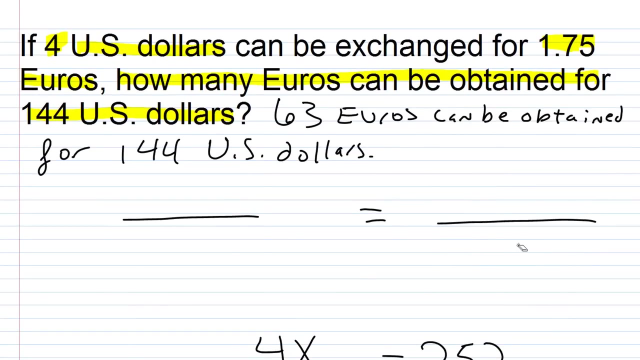 So this checks out. Now let me flip this and show you that it works either way. You just need to make sure that you have the same units in the numerator and the same units in the denominator. So let's say I would have taken and put euros in the numerator. 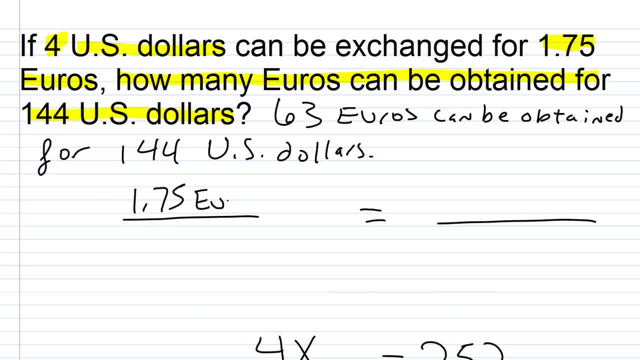 So 1.75 euros, And I put dollars in the denominator, 4 US dollars Over here. I just need to match that, So I don't know how many euros I can get. So that's going to be X euros. 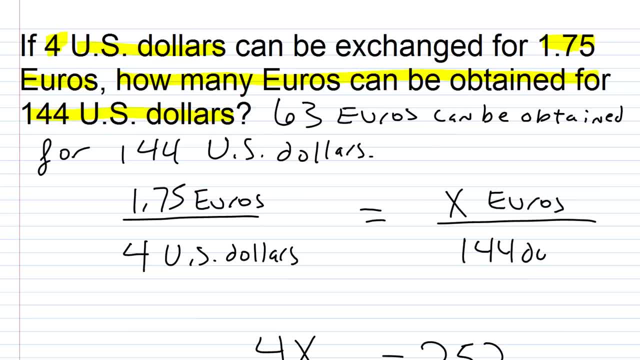 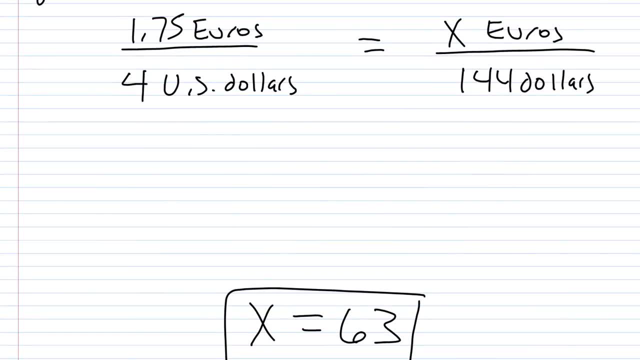 But I do know how many dollars. It's 144 dollars. So 1.75 times 144, again is 252.. And this equals 4X. And we know, when we divide both sides of the equation by 4, we get 63 for X, Right. 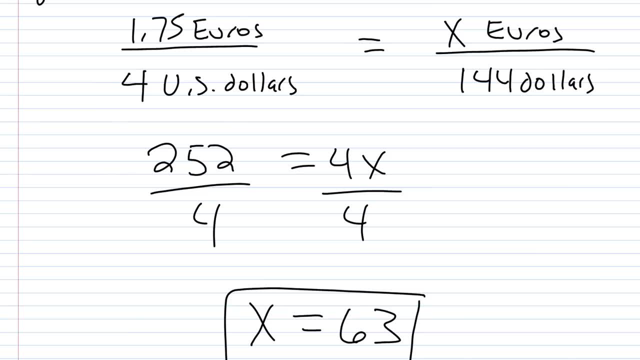 So X equals 63 either way. So I just wanted to show you that it only matters that you have the same units in the numerator and the same units in the denominator. If you mix it up, you're going to get the wrong answer.